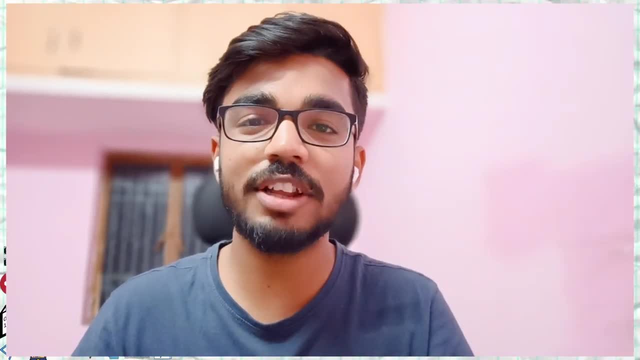 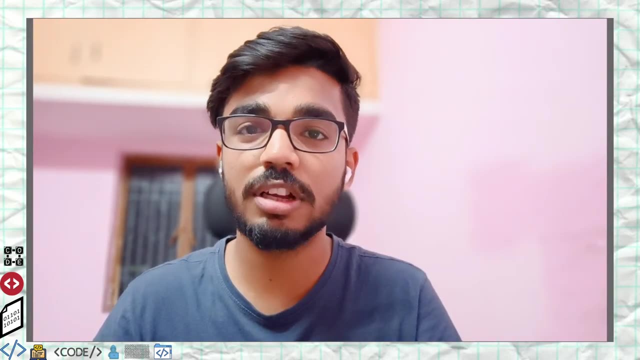 Hey everyone, my name is Tushar Jain and welcome to my channel. So in this video I'll be talking about proxy design pattern. What is proxy design pattern? then we will be writing code in Java to see how it works. So proxy is a structural design pattern that let you provide. 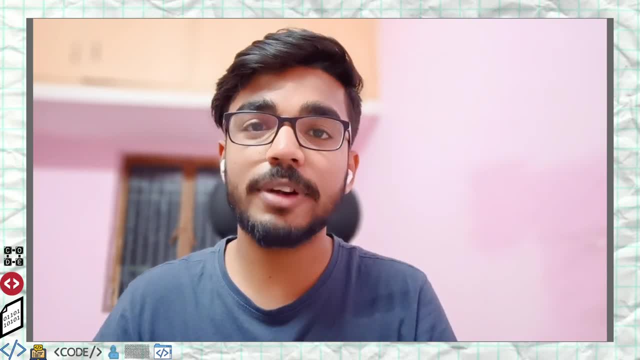 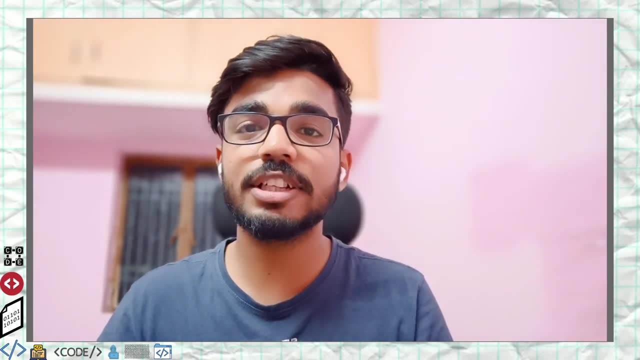 a substitute or placeholder to an existing object. But the question is why you want to create the substitute or a placeholder for existing objects. So the answer is: let's say sometime you want to perform something before or after the request gets to the original object, So in that case you can use your proxy design pattern. you can create a proxy. 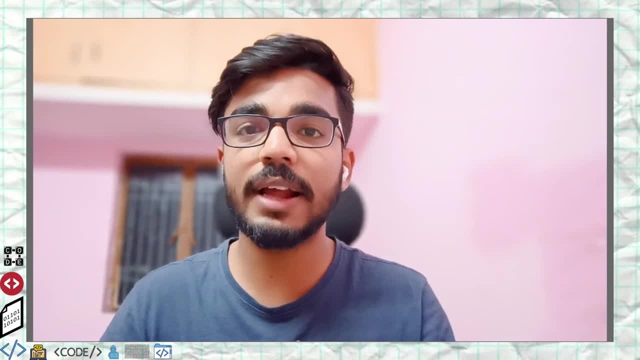 class for your existing class, existing object, and that proxy class will be connecting to the original class And you can perform something like you know: write, code or type some specific tasks before or after the call leads to the original object. This is the one use case. 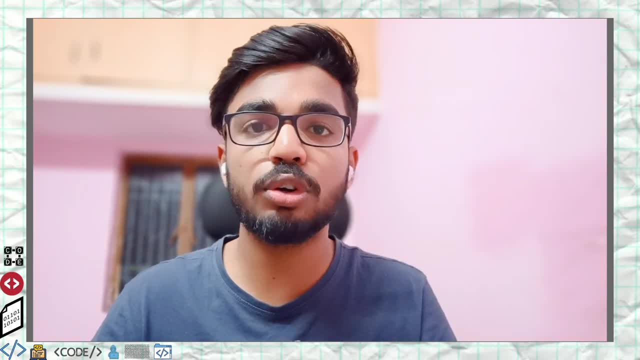 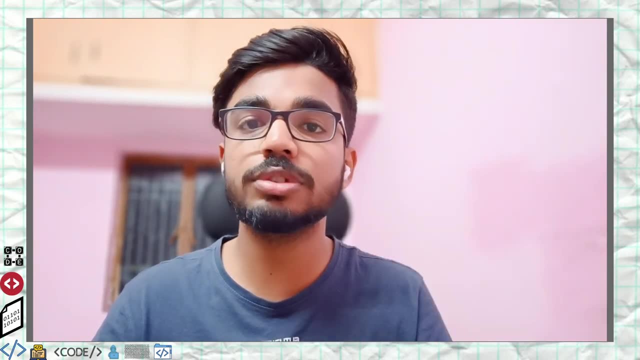 Another use case. let's say you have one massive object that consume vast amounts of data, vast amount of system resources, and you need to connect it to time to time because you need to use those functionalities. And to do that you can simply use the lazy initialization. 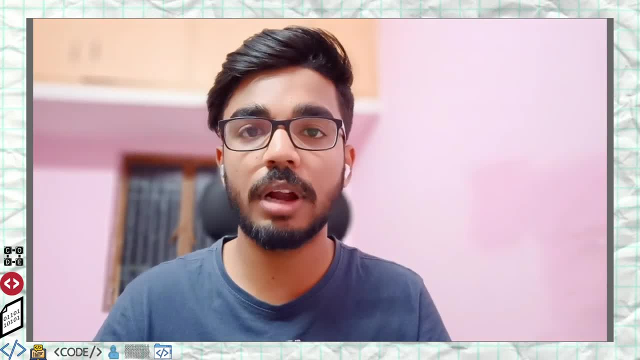 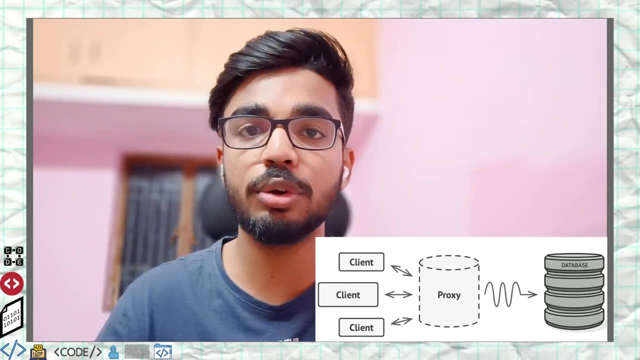 But there is going to be a lot of code redundancy because of this at client side, right? So in that case also, you can use a proxy class and put your code inside the proxy class and every time you want to connect to that service or object you can simply use the proxy class. 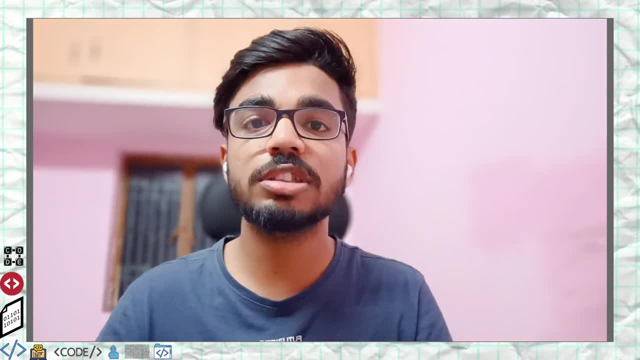 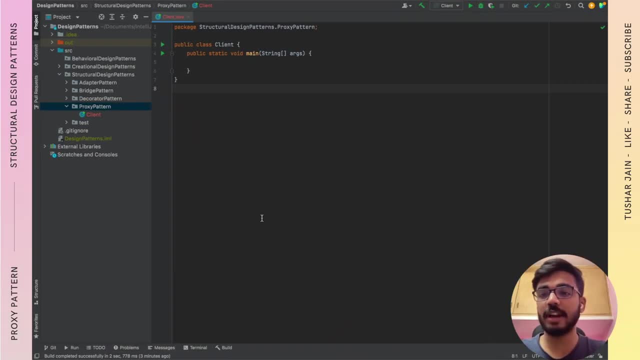 and also you can, in the proxy class again perform something before or after the call to the main object. Now let's jump into the code and see how it works. Let's write code for proxy design pattern. So I have created this client class which will be using the proxy. So first let's 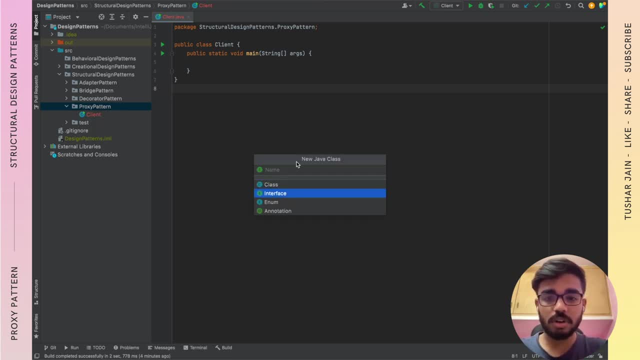 create one interface. We will call it database, or let's call it DB. Okay, so all the code is also available on the GitHub. you can go and check out the code if you want, And the link is in the description box below. And here first, we will create one method. we will 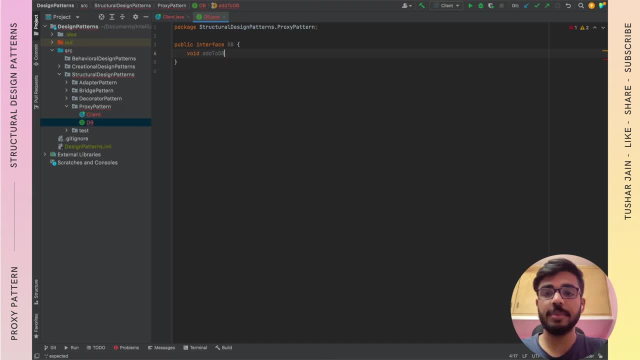 say add to DB, and it will simply take one string argument. Okay, so now we will create two class: first the main class, which we will call database, And then we will create one proxy class for this main database class and it will implement. 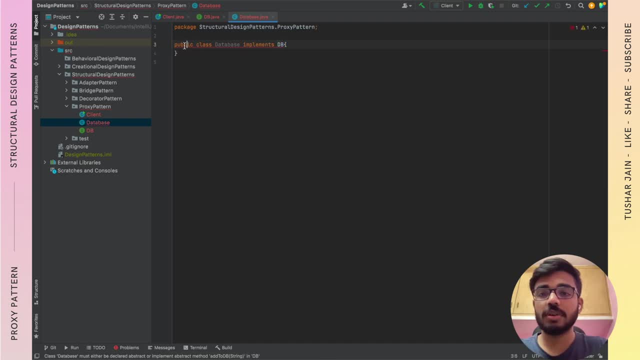 this DB interface, Uh huh, Okay. so, as we will say to now, we will just implement, define the methods which we have initialized in the interface. so we will simply say: so now, this is the main class. we can directly use this main class, but we want this to use via proxy. 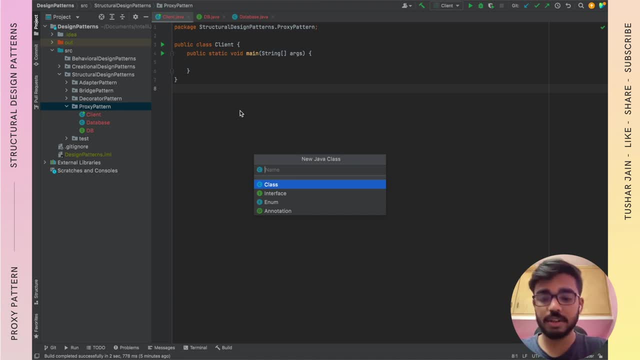 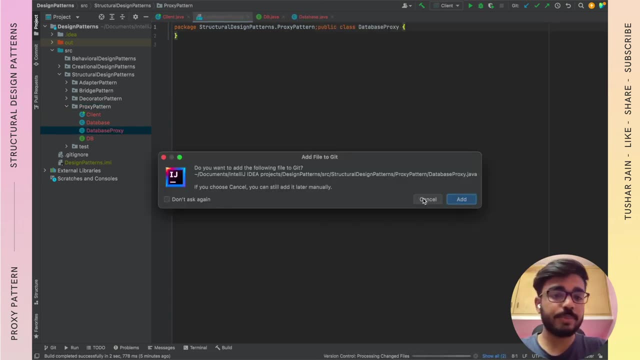 class. so for that we can create one proxy class, so we will call it database proxy and the database proxy and the DB. both will implement the same interface, so which, again, we will implement DB, and here we will just define the method in the interface. but before that we will create the object of this DB class, main DB class, and we will 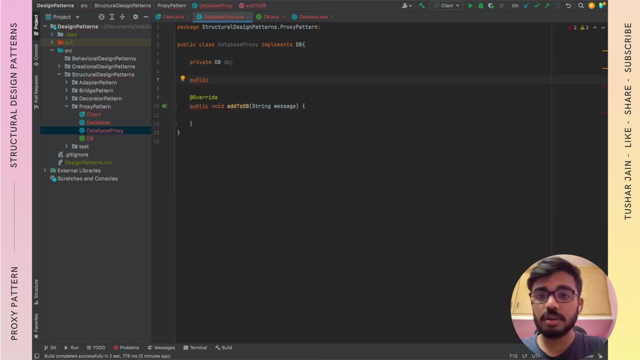 create the public constructor without any parameter which will initialize that this DB object. so now we will say this text: actually, let us say you see the header, click into the header file. we have told us this. we will say db dot, add to db and we will pass the message. but now in the proxy class we can do before or after anything. we pass to the database domain class. so let's say what you will do is, you will just change this string to math. let's say we will say message equals to messageto uppercase select. we have performed something beforehand, one after 2, также débierAnd similarly we can perform something after that. main2entebl di byo3al bar overda the https file. 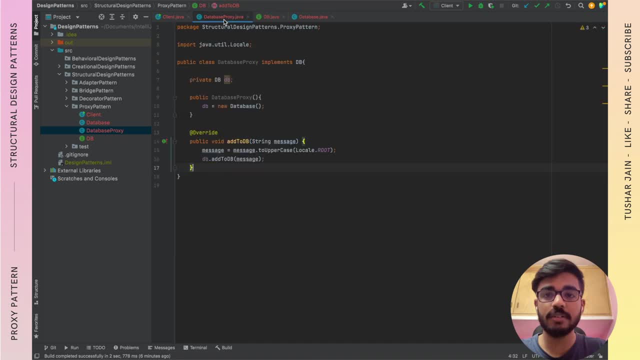 functions: main function executed in the main class, in the db class, so we can add that code here. so now let's use the client and create the object of db, of the database proxy. we'll say: database proxy equals to db, equals to new database proxy, oh sorry. and then just db will call add to db and let's say we will say: 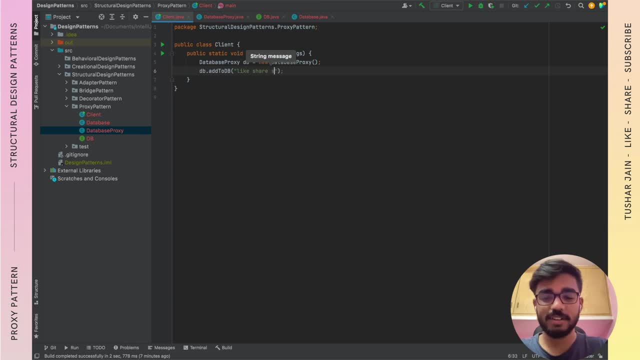 like share, subscribe, and now, if i will run this class, so this is all in lowercase and it is added into the uppercase and it is added into the db. so this is how we can use proxy class to. so this is how we can use proxy class to.